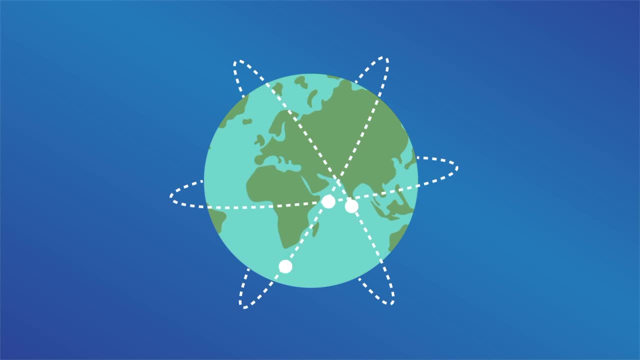 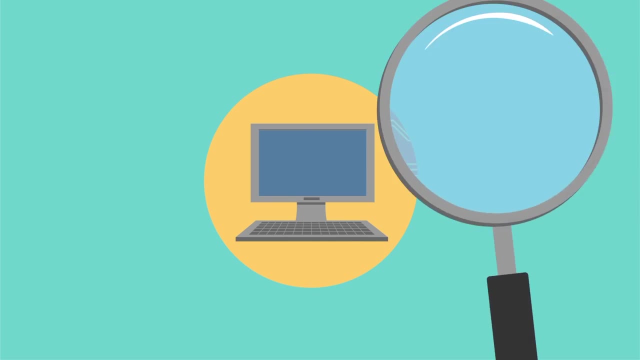 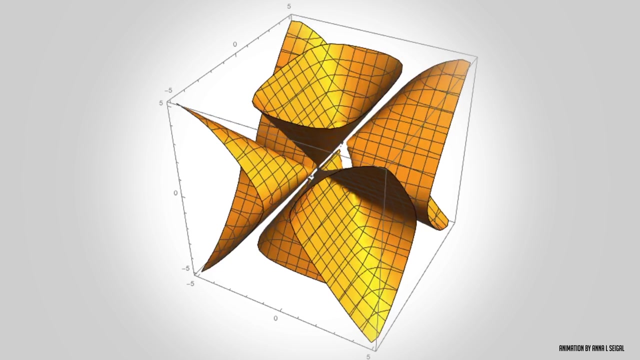 better at understanding the complex non-linear relationships that govern both natural phenomena and social systems. These are not just abstract notions anymore. Dig deep enough into almost any problem and you'll find insight. in the language of mathematics, Solutions to these problems will rely on mathematical methods from these fields too. While algebra, geometry and topology have 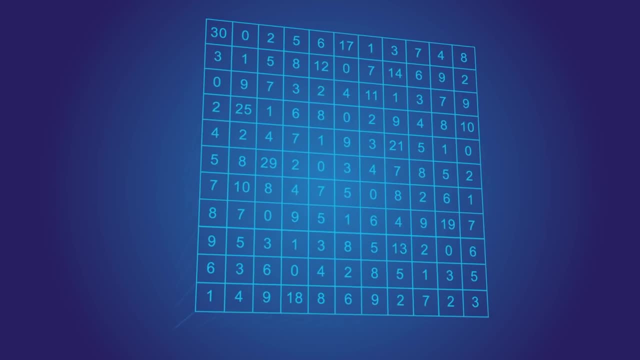 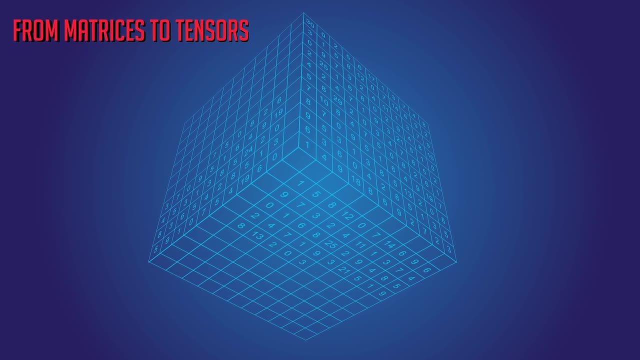 long been studied theoretically in academic contexts. the past decade has seen an explosion of applications As applied. algebra and geometry continue to grow and change. many of the theories that have been studied in the past decade have been studied in the past decade. The theories that power those applications are still waiting to be discovered and described. 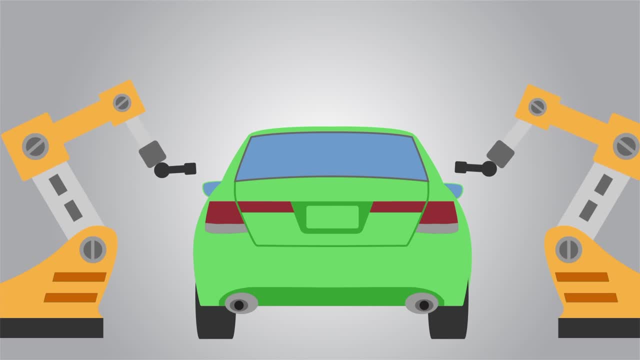 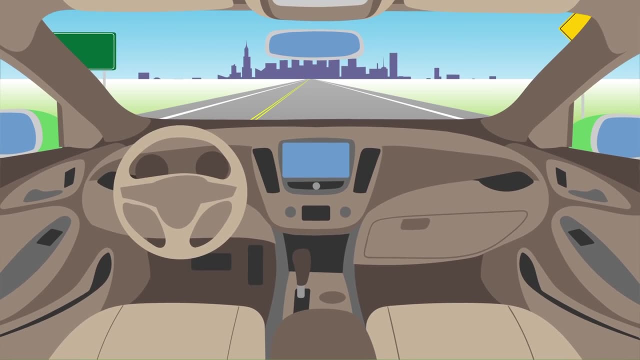 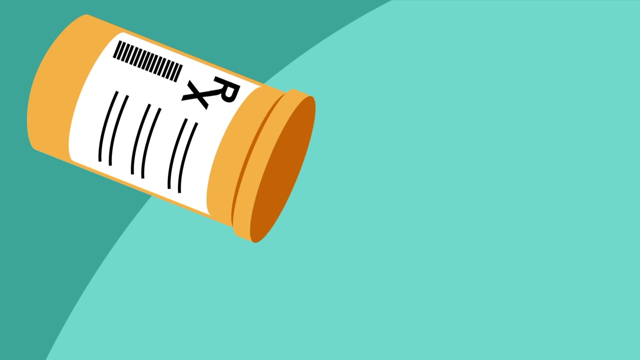 For example, today, control theory powers the path a robot's hand takes as it installs a car part on an assembly line. Tomorrow, algebraic geometry will drive the computer vision that allows your car to merge itself onto the freeway. Today, experimental design outlines the best way to 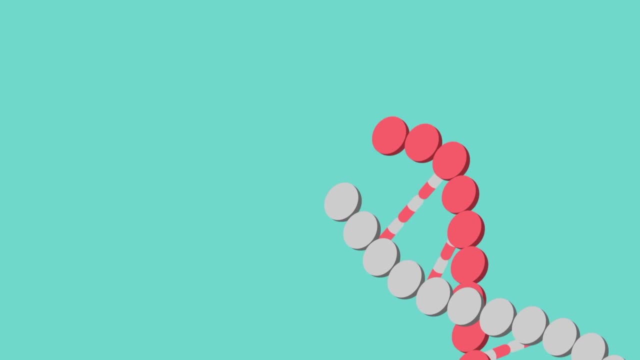 conduct drug trials. Tomorrow, algebraic topology will show how gene regulatory networks influence the causation of disease. Tomorrow, algebraic topology will show how gene regulatory networks influence the causation of disease. Tomorrow, algebraic topology will show how gene regulatory networks influence the causation of the. 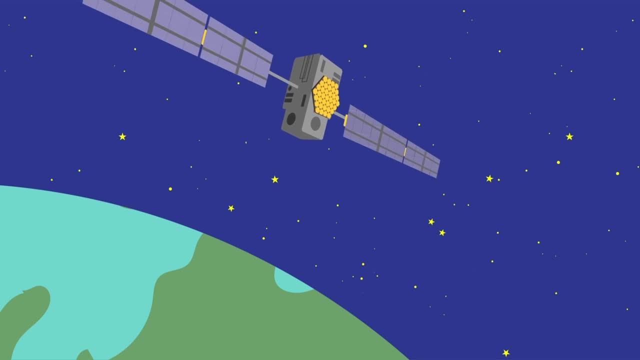 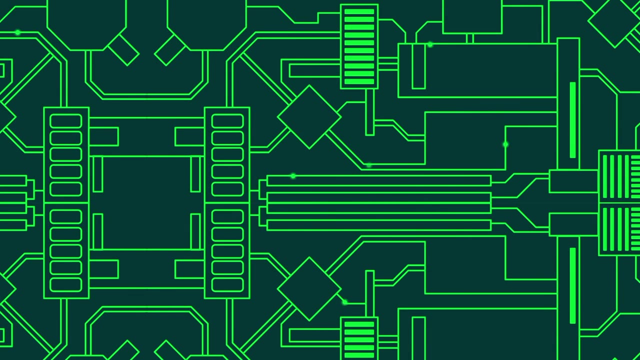 diseases those drugs are meant to treat. Today, dynamical systems show how satellite solar panels can fold into rocket cargo bays. Tomorrow, tensor networks govern the physics of the quantum computers inside them. Mathematicians do amazing things. They discover beauty hidden in the. 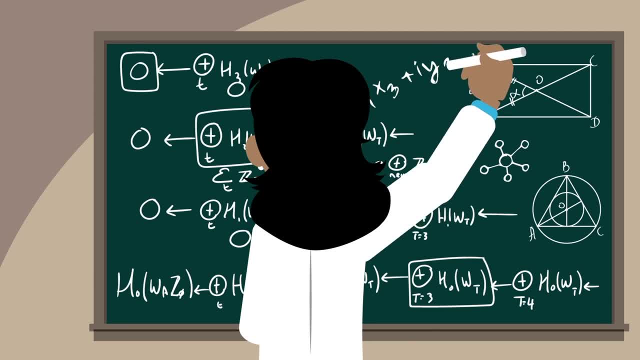 natural world and come up with ways to change that world for the better, As the fields of algebra, geometry and topology increasingly move from linear to nonlinear and from theory to practice. algebra, geometry and topology increasingly move from linear to nonlinear and from theory to practice. 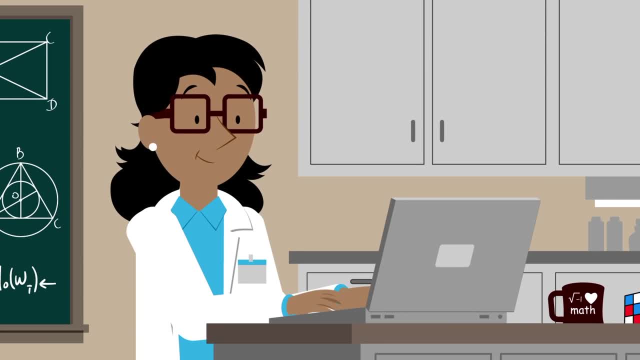 algebra geometry and topology increasingly move from linear to nonlinear and from theory to practice. you can be a part of that transformation. If you want to see these methods address problems of the real world, you have a new home. There's now a journal that connects algebra geometry 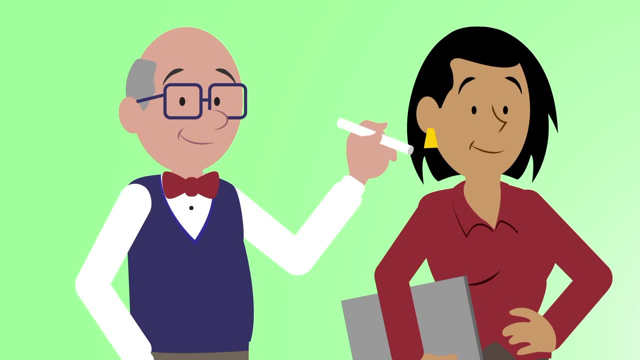 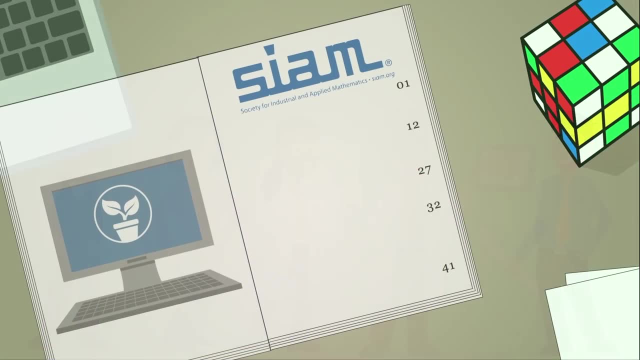 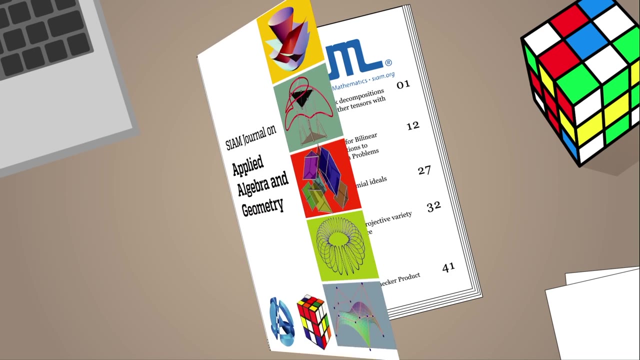 and topology to applied mathematics. Join fellow mathematicians, computer scientists, geneticists, neuroscientists and engineers. Share your theories, your experimental data, your code, your graphs and graphics all in one place. Welcome to the Sci-Am Journal on Applied Algebra. and Geometry.